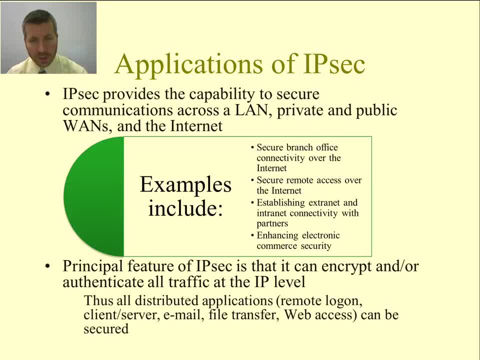 As an internet standard. here are some of the applications of IP security. It allows us to secure communications across a LAN, private and public wide area networks and also the internet. Just some examples here from our textbook: secure branch office connectivity over the internet so that they're able to communicate back with 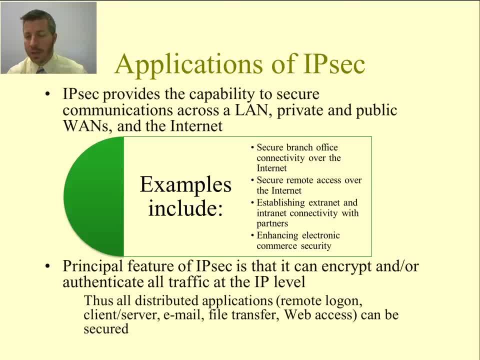 let's say a corporate office- secure remote access over the internet, establishing an extranet and intranet connectivity. The principle feature is that it can encrypt and or authenticate all traffic, and it's doing it at Layer 3.. It's doing it at the IP level instead of doing it at some of the other levels. 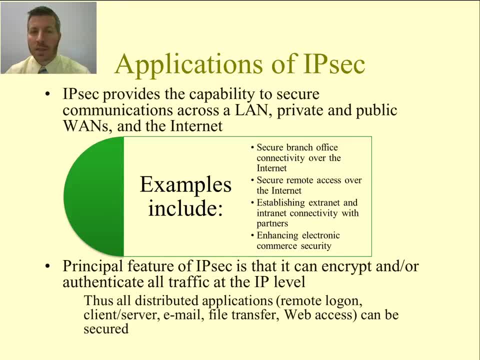 If you look back to the different encryption algorithms that we've discussed so far, those were all running at Layer 7.. When we're using RSA or triple DECs or AES, these are all running at Layer 7. So everything below that is still going to be unencrypted. 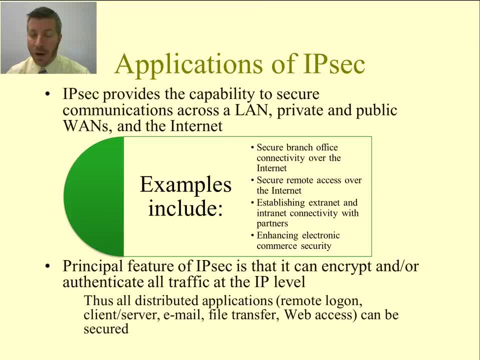 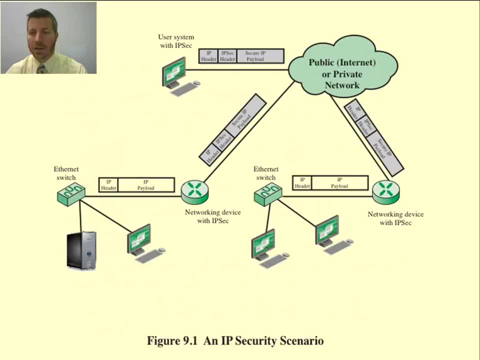 IPsec is where we're now going to look at encrypting at layer 3 instead of waiting until we get all the way up to layer 7.. Here is an overview of how it works, So starting up at the top. you see, this is a user system that has IPsec in it. 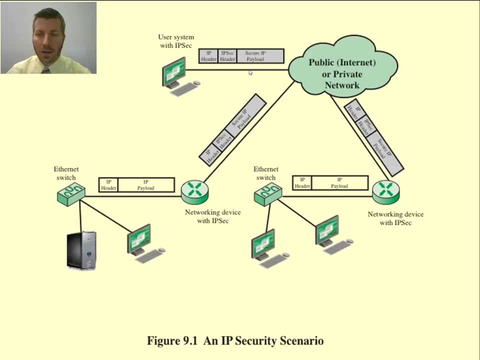 Now, when it sends off the packet, we still have the IP header at layer 3, but then we have an IPsec header. This is the IP security header, and then we have the secure IP payload. Now, inside of the payload of an IP packet is a segment which is from layer 4.. 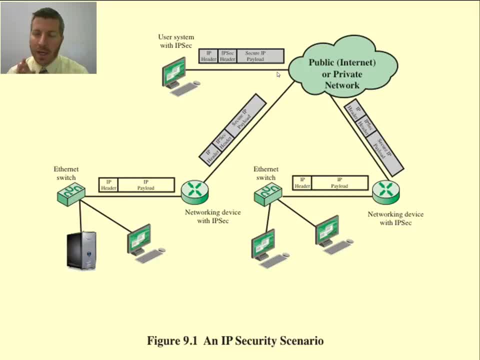 So, if you remember that, we keep wrapping from each layer, so the user types something that becomes the message goes into our layer 7 message, Then we go down through the layers, layer 6, layer 5.. In the Internet of course we don't have those two layers. 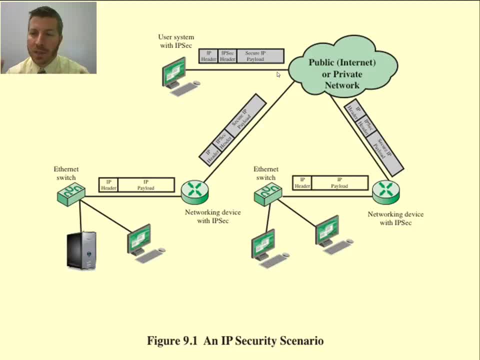 but looking at the OSI model, we go through layer 6, we add a header and the payload becomes the layer 7 message. At layer 5, we add a header and then the payload becomes what we got from layer 6.. 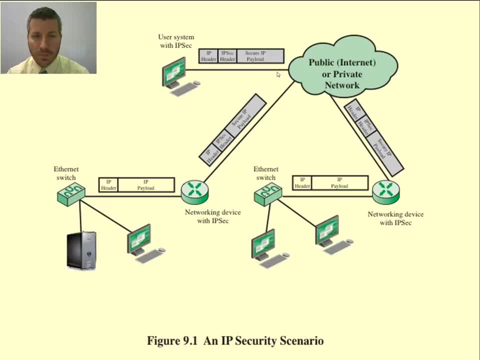 We go down to layer 4, and at layer 4, we have a segment, so we add a header onto it and the payload becomes what we got at layer 5.. Then we go down to layer 3 at the IP layer, and at layer 3, we add the header. 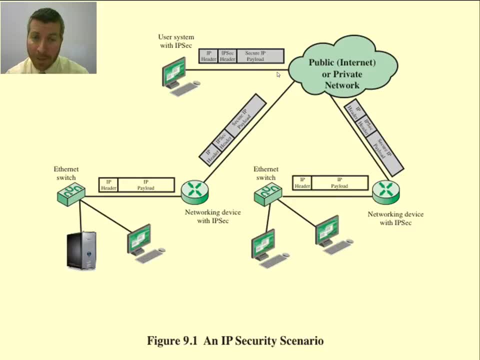 and the payload of an IP packet or of a layer 3 packet is going to be your segment. So what we've done now is we've secured the segment as the secure IP payload. So this is now going to be encrypted for us. 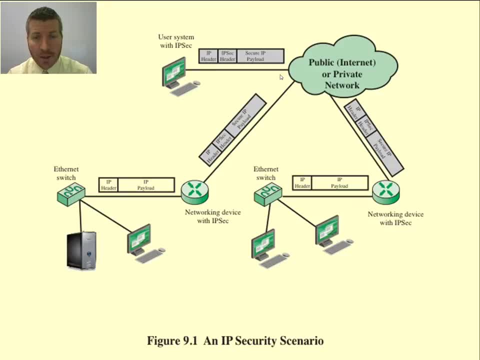 And so the only thing that's unencrypted now is the IP header at layer 3.. And below that then we also have layer 2, which is going to be unencrypted, And layer 1,, of course, is not encrypted. but this is just the bits. the voltage, layers, levels. 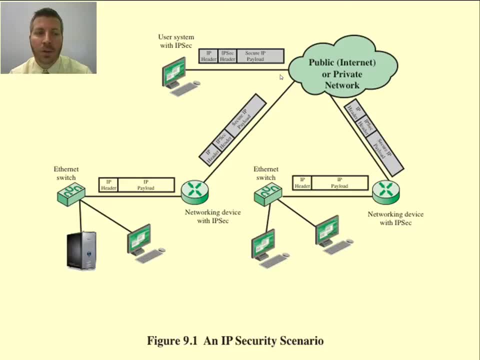 the bits that are going across the wire. So that's not going to be encrypted either. So we've encrypted down a much lower layer. We still had to keep the IP header the same, though. If the IP header wasn't going to be the same and we actually had just the IPsec header. 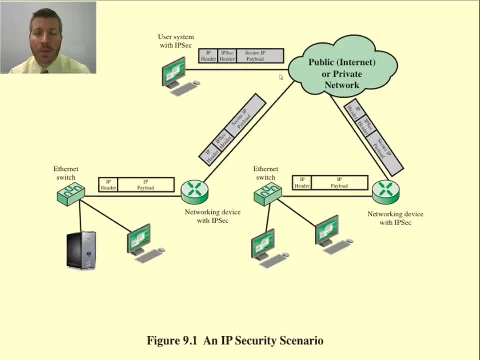 the problem that we would have there is that every router throughout the Internet would have to support IPsec, And this is not something that's going to happen anytime soon. IP version 6 supports IPsec. However, we have to make sure that we're supporting both. 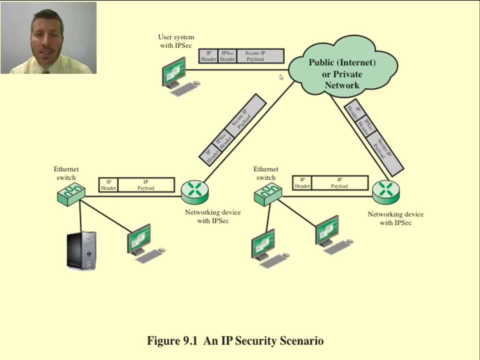 IP version 4 and IP version 6 simultaneously, since there are so many routers already in existence on the Internet that support IP version 4.. So what we have to do is we still have to have the IP header, so that all of those routers in the Internet are still going to be able to route our packet and get it to the desired destination. 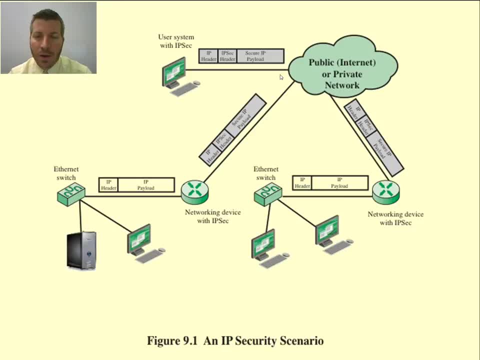 However, everything above layer 3 is now going to be encrypted, Actually not even above layer 3.. This is everything other than the header at layer 3.. So the payload at layer 3 and everything above that is going to be encrypted now. 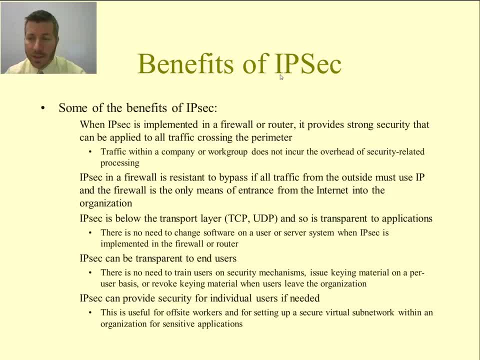 Okay, So some benefits that we have to IP security. Obviously, we have strong security when it's implemented in a firewall or a router for all traffic which is crossing the perimeter. IPsec is below the transport layer, so it's below the TCP, UDP, which both run at layer 4.. 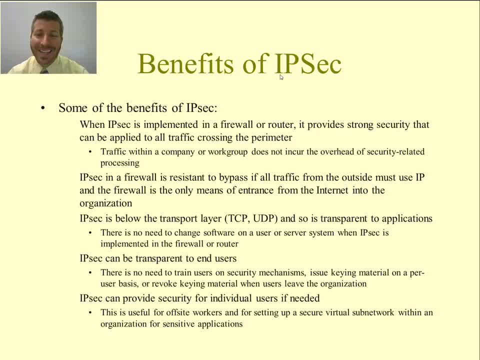 So it's transparent to application. We are going to decrypt this before we send the data back up to layer 4, so the end users don't even necessarily have to know that we are using this because, remember, layer 4 is the first end-to-end layer. 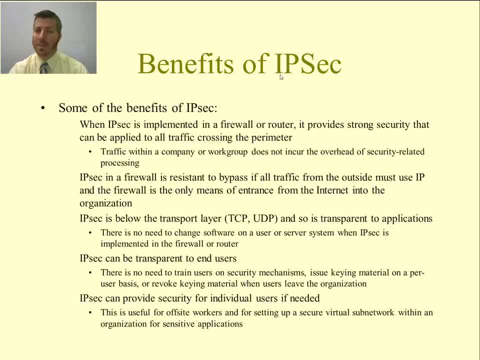 That's an important thing to note about layer 4, that it's the first end-to-end layer that we have in the OSI model. If we're encrypting the payload of a layer 3 packet, then layer 4 is not going to know about it because we're going to decrypt the payload. 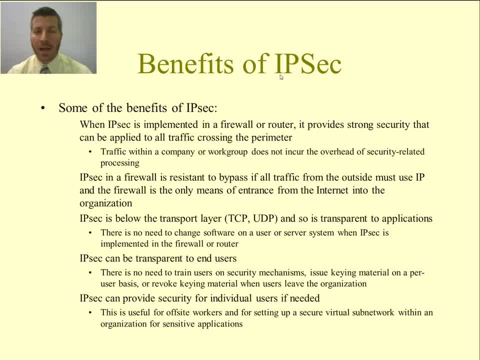 Okay, So we're going to decrypt the payload of the packet before we even send that back up to layer 4, so layer 4 doesn't need to know about it and makes IPsec transparent to applications, meaning we don't need to change any software that we have on user or server systems, and that's a big plus here that we can have security, but we don't need to change anything on every single end-user's computer. 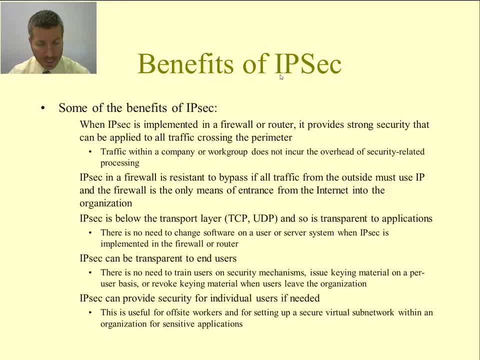 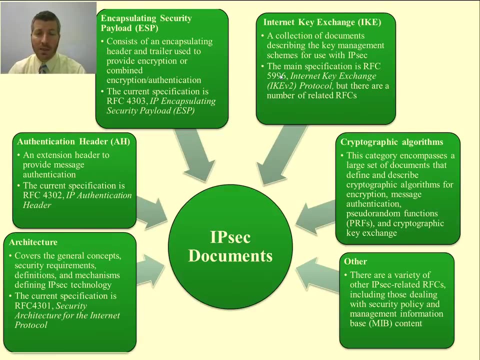 That covers the next point. there also, and IPsec can provide security for individual users if needed. This is useful especially for setting up secure virtual subnetworks, so virtual networks within an organization also. Here is a diagram. There is a number of different documents that have to go into creating an IPsec packet. 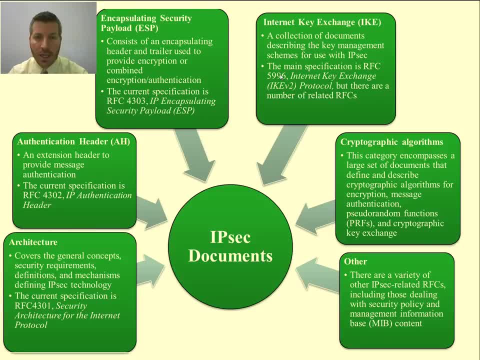 You see, starting down at the bottom left, the architecture covers general concepts, security requirements, definitions, mechanisms, defining IPsec technology. they show their RSC 4301.. Okay, Moving up, we get to 4302, the authentication header. 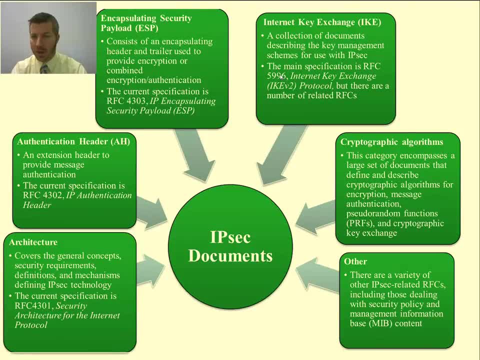 It's an extension header to provide message authentication Up at the top. encapsulating security payload consists of an encapsulating header and trailer used to provide encryption or combined encryption and authentication. We've talked about encryption. we've talked about authentication in the past. 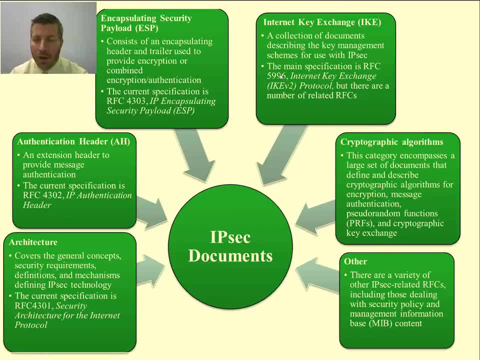 Hopefully you understand the distinction between the two of those comparing who's able to read the data, as opposed to making sure that the data came from the person. Okay, Okay, Okay. Hopefully you understand the distinction between the two of those comparing who's able to read the data, as opposed to making sure that the data came from the person from whom we believe it should. 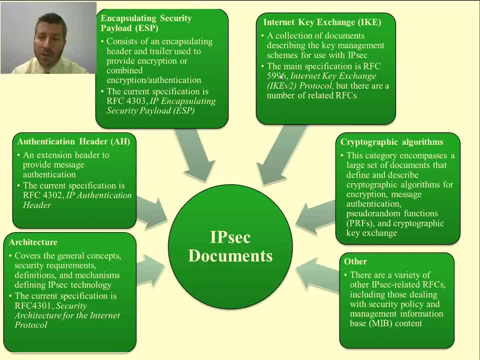 Okay. Internet Key Exchange- Collection of documents describing the key management schemes for use with IPsec. We've talked about key management schemes before. How do we get a key from one computer to another, especially when we're dealing with symmetric key encryption And then cryptographic algorithms? 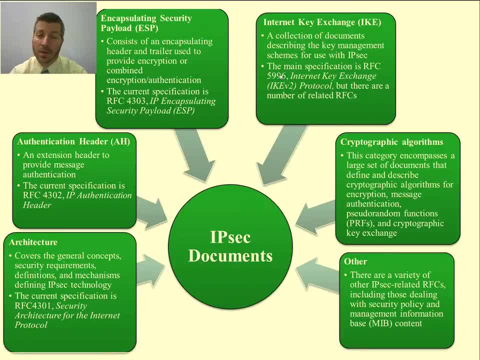 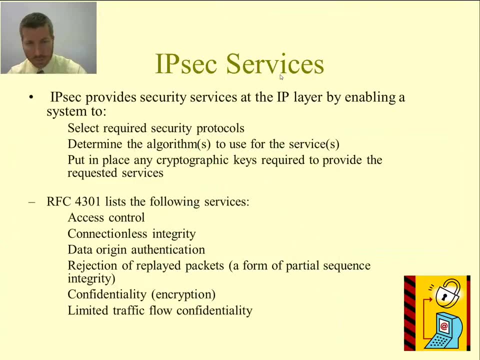 We talked about a number of different cryptographic algorithms and this is an open algorithm where we can use this, use whichever cryptographic algorithm we wish for. We use JSON, JSON, DNS, bind and a lot of similar ones. would like Okay, some of the services. security services at the IP layer enables the system to 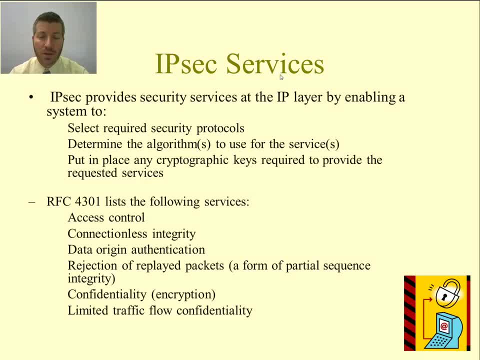 select the required security protocols, determine the algorithm to use for the service, put in place any cryptographic keys required to provide the requested services. This is what I was just talking about: that we have this open that we are able to use whatever we would like there. 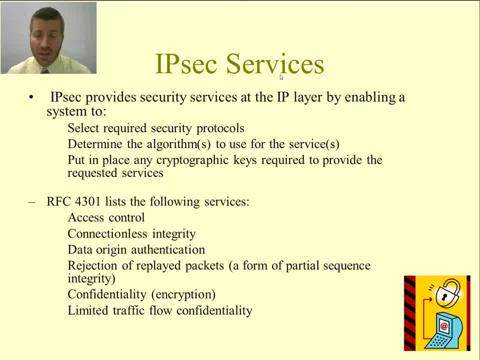 RFC 4301 lists a few more services. You can take a look at that RFC. I wouldn't recommend doing this while you are going to sleep at night, unless you have insomnia and would like to. But we have access control, connectionless integrity, data origin authentication and so on. 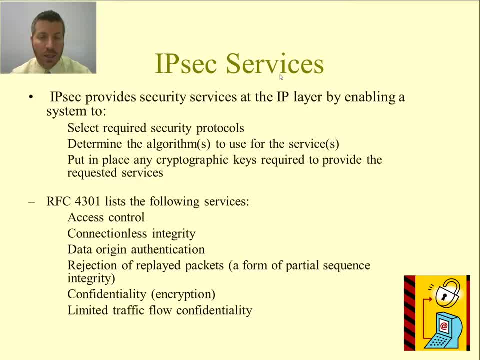 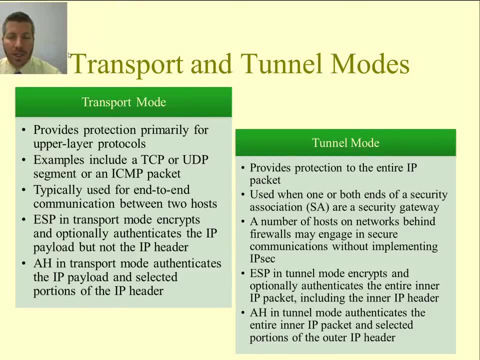 Rejection of replayed packets, confidentiality and limited traffic flow confidentiality. There are two modes that we have: transport mode and tunnel mode. This just gives an overview of what the differences are between the two. Transport mode provides protection primarily for upper layer protocols. 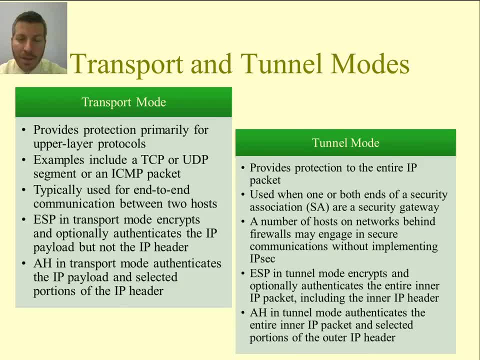 Examples include a TCP or UDP segment or an ICMP packet. This would be transport mode. This is kind of what we've described so far, used for end-to-end communication between two hosts. Tunnel mode, on the other hand, provides protection to the entire IP packet. It's used when one or both ends. 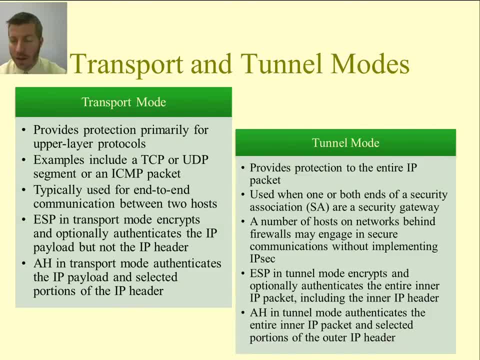 of a security association are a security gateway. But what we are able to do here then is that if our entire network, let's say, is behind a firewall and we have our entire network that supports IPsec, then maybe we don't even have to have that IP header on the front, But instead we can encrypt the 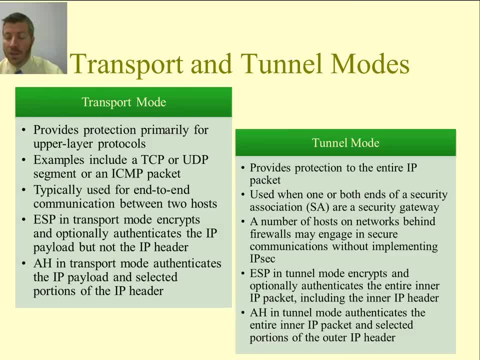 entire IP packet and just have the IPsec header rather than just the IP packet. So that's an interesting idea there that we can get away. and then people wouldn't even be able to see who we are trying to speak with, the destination of the packet, if we were able to encrypt the entire.